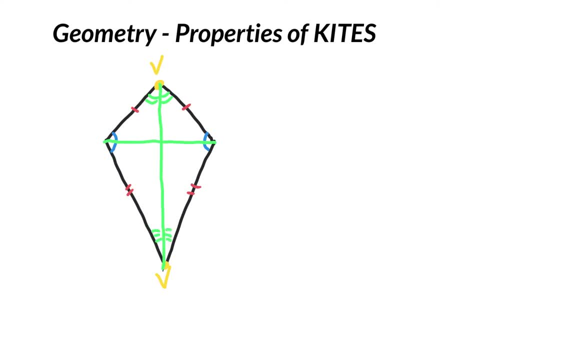 and these two are equal. Now, they may not necessarily be equal to each other across the kite, but they bisect. that diagonal bisects the angles. Next property is that this bisector, the one from vertex to vertex, bisects the other. Guess I better. 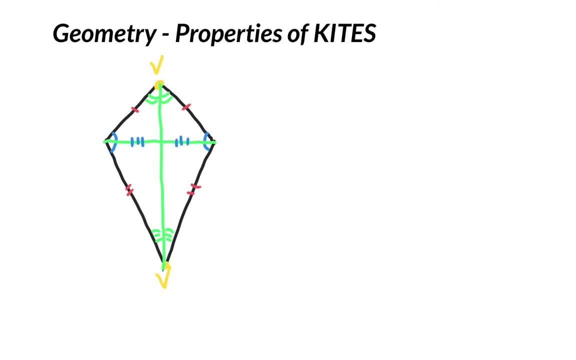 put three in Bisects, the other diagonal, and finally this bisection makes a 90 degree angle. There's a right angle there. Let's write all of these down, Alright? so let's just point these out. Two pairs of adjacent, congruent sides. So this pair. 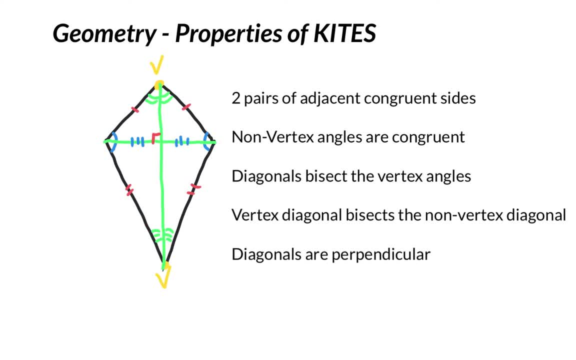 and this pair and again, unlike a rectangle where the congruent sides are across From each other, these two actually meet. Where they meet, so these two meet, is a vertex angle, and these two meet is a vertex angle. The non-vertex angles are congruent, So this angle and this angle, The diagonals bisect the vertex, So our 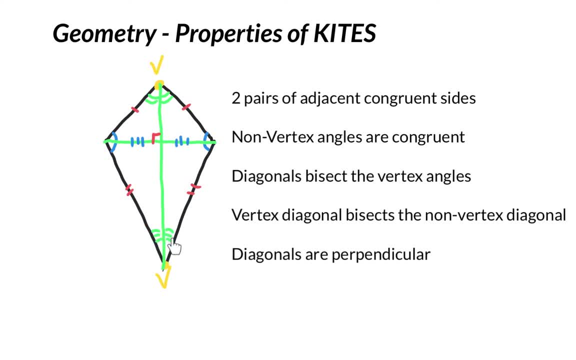 diagonal here, from vertex to vertex, cuts the angles into equal to equal angles. Okay, the vertex diagonal bisects the non-vertex. So this one vertex to vertex cuts this one into two equal pieces, and the two diagonals are always perpendicular to one another. A lot of times it's very evident by the picture. 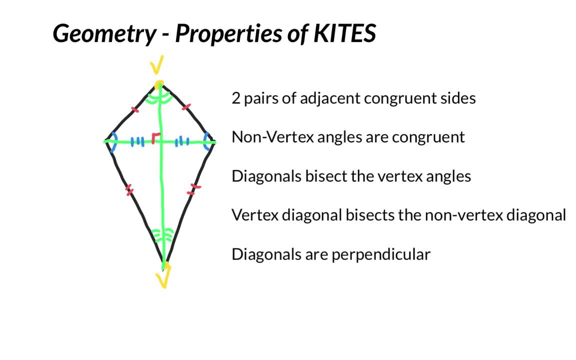 and kind of drawing a kite like the kind of kite you'd fly kind of leads you to all of these things, but these are the big properties that make a kite. If this video helped you, please like and subscribe for more geometry help. Thanks for watching.